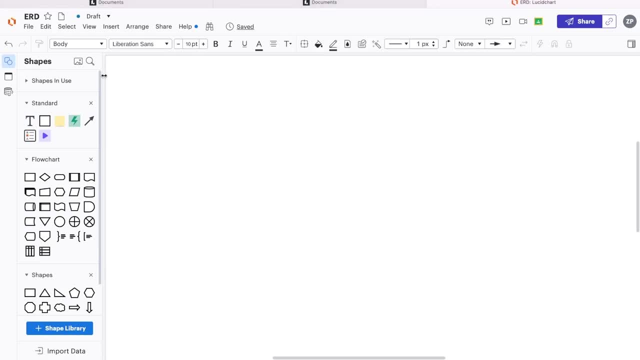 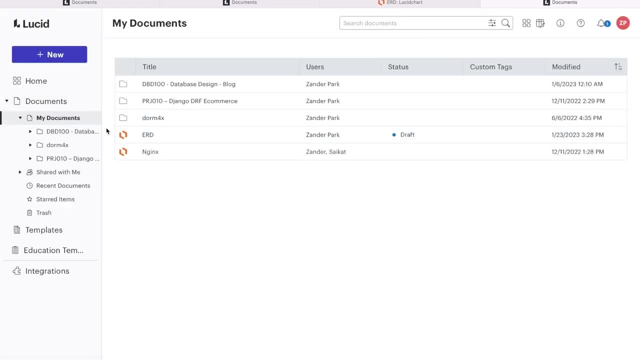 up multiple tabs. You can already see I have three tabs open here already Now. if I click on this option here, that'll take me back to the documents Now. by default, a new file will be stored in the root of my documents. I can go ahead and just drag that. 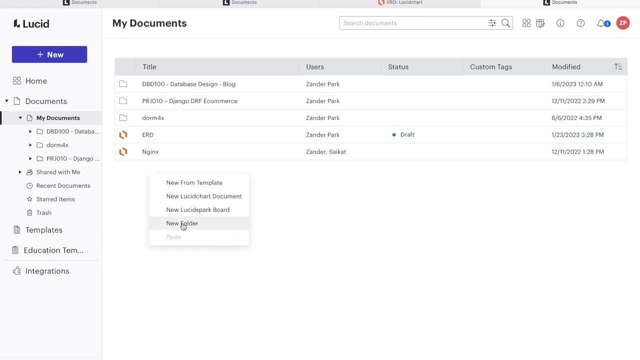 into a folder if I need to. I can right click create a new folder if I want to, or click yeah, create a new folder. in this way, If I select new, for example here, I can also select a folder. 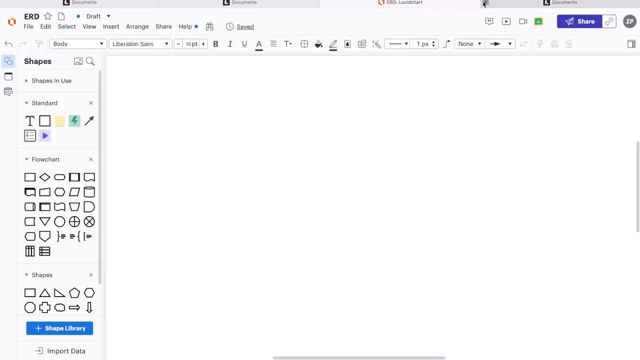 as well. Okay, so back to this tab. I'll just remove the old tab, The entity relationship diagram or entity relationship model. So this is a graphical representation of, in this project, our database. There aren't many symbols or shapes that we need to learn. 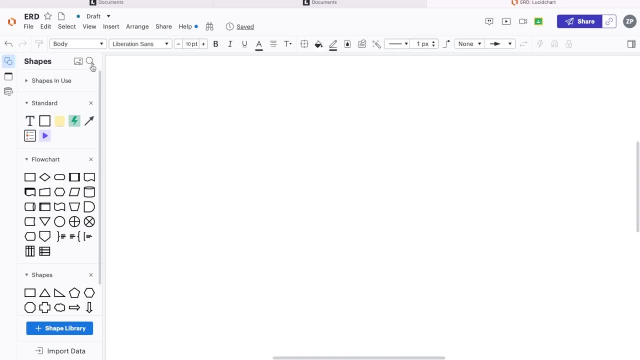 In actual fact there are probably three or four. So to access these shapes, we can go ahead and select shapes here and type in ERD. That will bring up some shapes. So you can see there are multiple ways of representing an entity. So depending on your preference, 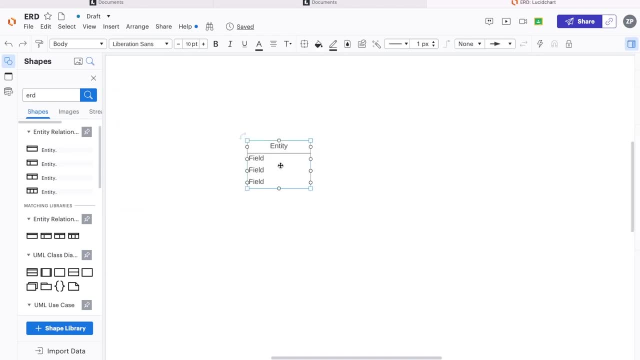 will depend on which one you select here. but let's just go for the basic entity shape. So I'm going to zoom in a little bit here. So if you want to zoom in, I've used the command button and my mouse, but at the bottom right you can't see it on my screen. At the bottom right hand. 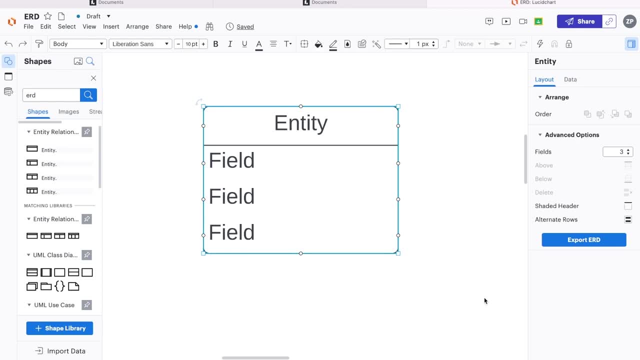 corner there is a zoom level, zoom options. So from here I can select the name of the entity, person, and then the attributes. I can double click there. That will give me access then to create some attributes, So for example first name and so on, And then I can control the amount of. 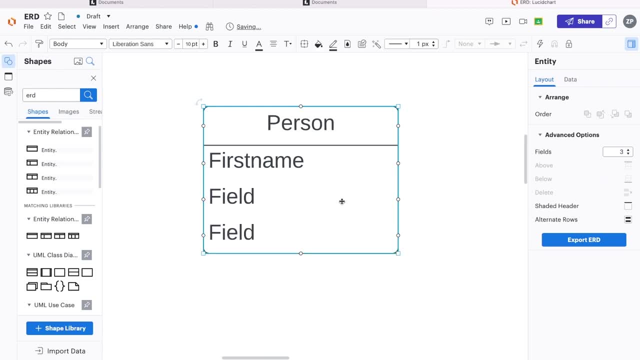 fields. I have a utilize field, I have a use field and I have a use field, So I can control the amount of fields. So I can control the amount of fields. So I can control the amount of fields- This option here on the right hand side when I select my entity, or I can double click. 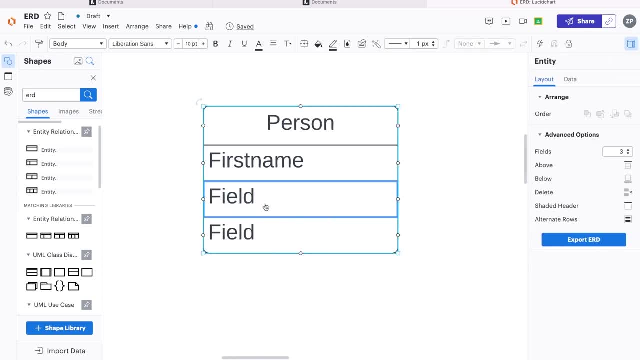 or actually just single click, get the field to be highlighted, right click and then delete the row and insert new rows above and below. So the main component of the entity relationship diagram is the entity. That's what we have here, But this is an entity relationship diagram. So 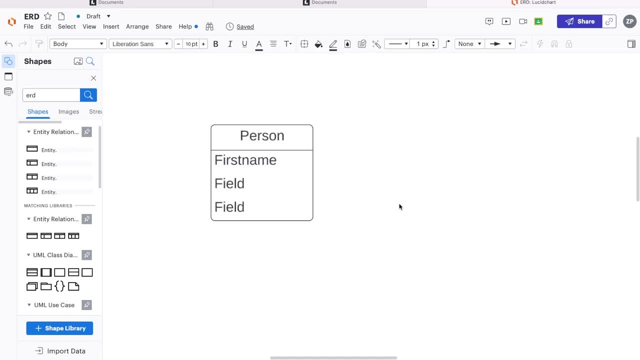 this is suggesting that there are relationships between the entities. Apologies there. So what I can do, let's just go ahead and just copy and paste this And let's just rename this something different, for example, car, And then let's give the car. 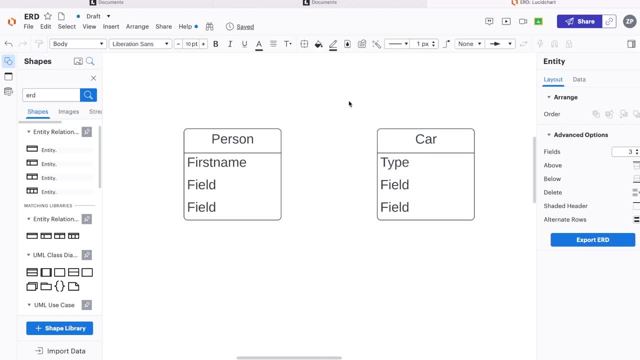 a type, Right? so we want to build a relationship between two entities. Now in this tutorial I am not going to explain how to determine relationships, just show you how to actually depict a relationship between two attributes. So generally here, when we're developing databases, 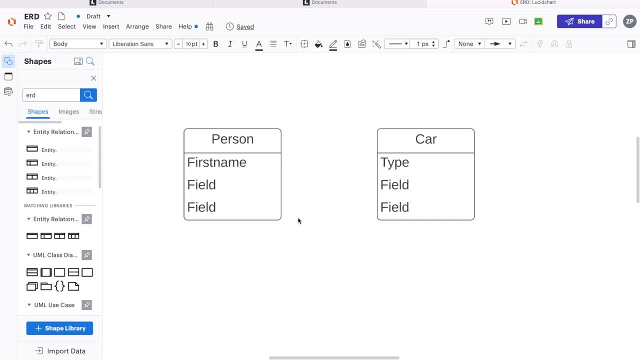 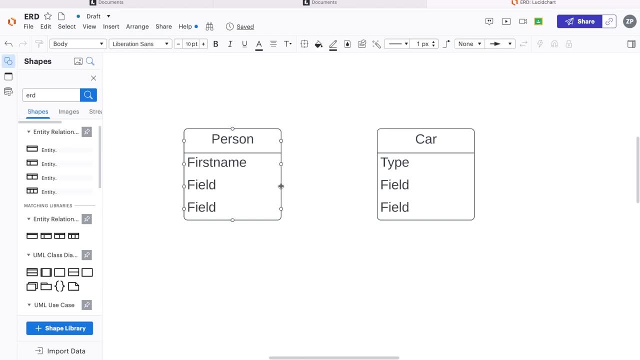 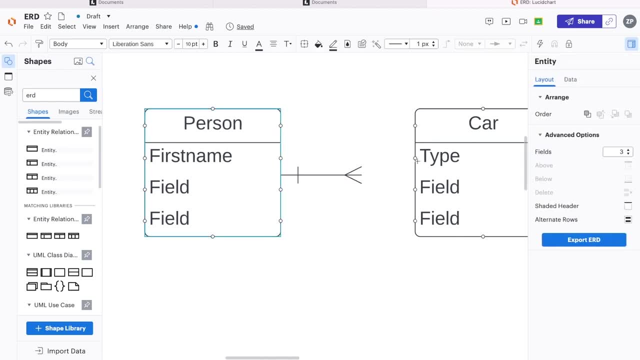 that appears. So that just tells me that I can press my mouse down or your touchpad, whatever you're using, keep it pressed and then drag and then create this new relationship. So what I've done here is I've created this default relationship And the default relationship. 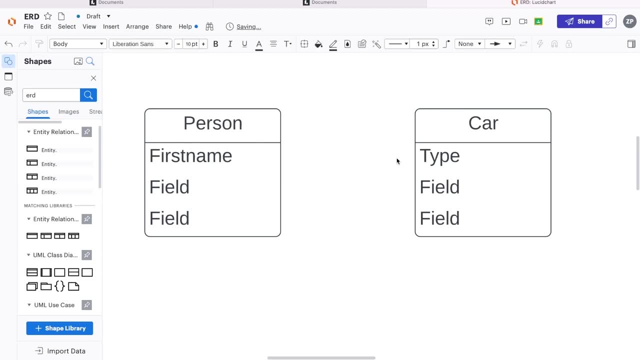 is a one to many, So let's just go ahead and do that. So let's just go ahead and do that. So the one is always going to be on the side where I dragged from. So notice, this time I dragged from the other side. the one component here of the relationship is on the right hand side. 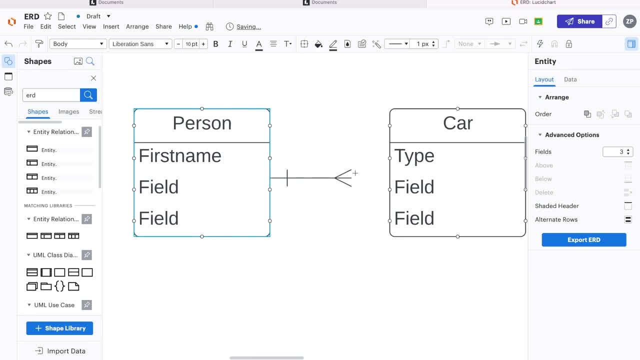 So it doesn't matter, because we can go ahead and actually define that. So if I make a new relationship, define a new relationship between these two entities. up the top here I've got a few tools where I can then change the end symbol or the end shape. So, for example, here I've now 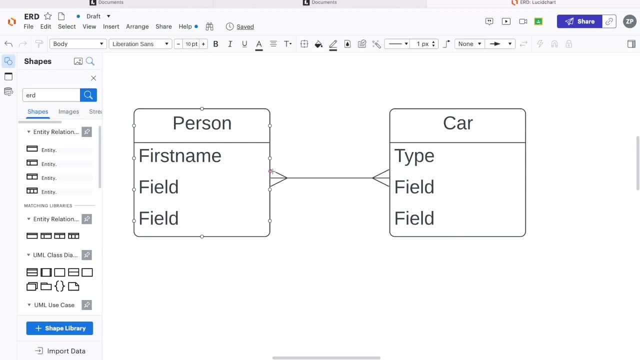 created a many to many, So let's just go ahead and do that. So let's just go ahead and do that. So the crow's foot here defines a many relationship. So I'm saying here that the person, for one person, is connected to many cars, And for one car, a car might be associated to multiple people. 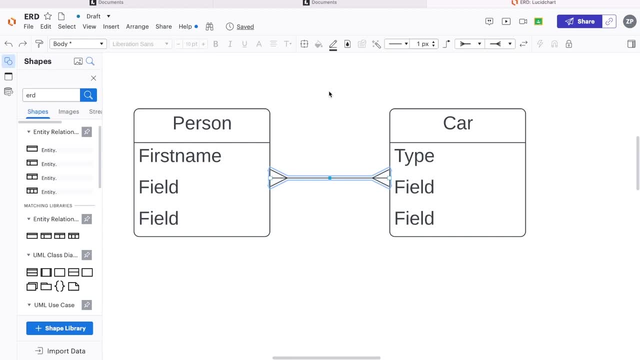